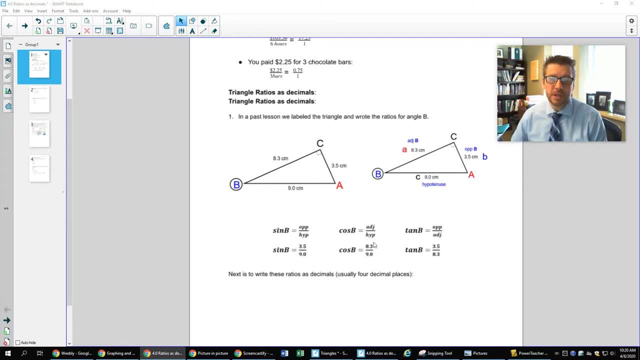 now that sine ratio is opposite over hypotenuse, cosine is adjacent over hypotenuse and tangent is opposite over adjacent. And there are other ratios in these triangles, But these are the three primaries And these are the ones that we usually work with. So our first lesson was just about 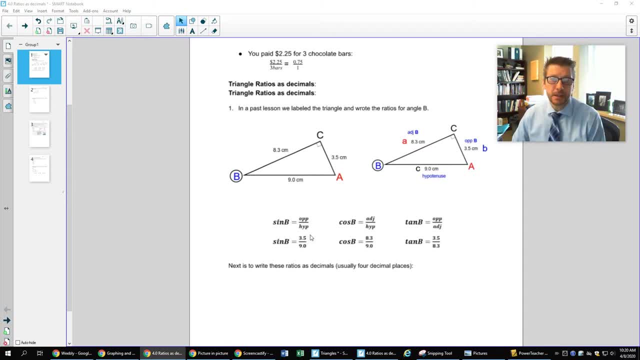 writing ratios And, like I said, ratios for us in the past lots of times are fractions And we just want to know that when you write a ratio you can actually change All three of these ratios to decimals as well. So sine of B would be three and a half divided by nine. 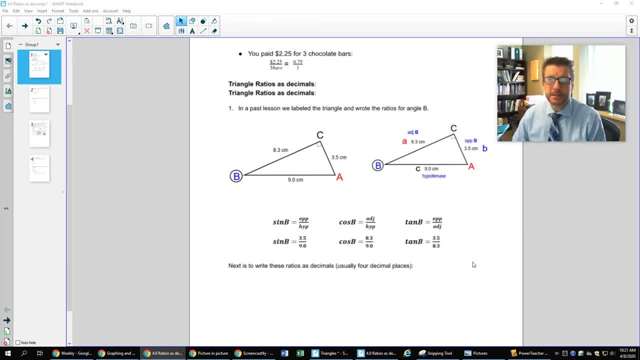 Cosine of B would be 8.3 divided by nine, And the tangent of B would be three and a half divided by eight and a three. And if I did all that work I could then say that my sine cosine and tangent 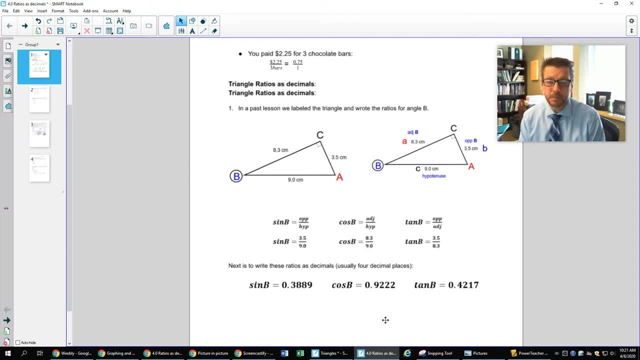 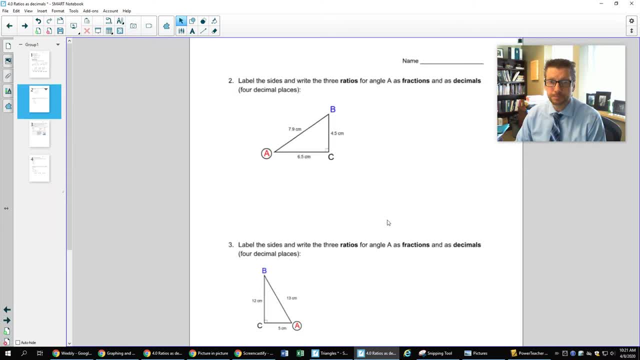 going to use trach, And then we're going to use trach, And then we're going to use trach, And then we're again practice doing some decimals. so here again we've got a angle a and we want to again just review how do we name angle a? and we want to again talk about the idea that we have. 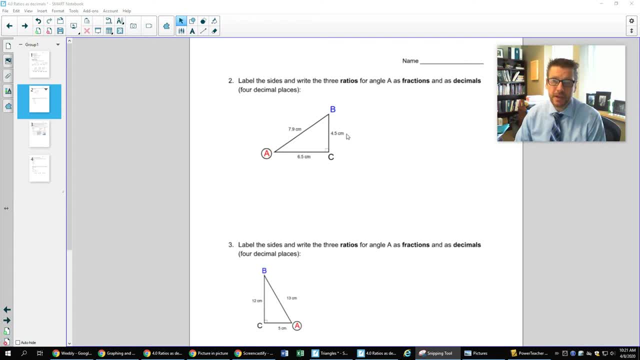 opposite of a. so big a opposite of a will be four and a half c, 90 degrees. this will be the hypotenuse. so if i have opposite and hypotenuse then i know i want to have adjacent. so i'm just going to grab another diagram from over here and i'm just going to fill in our, our labeled triangle. 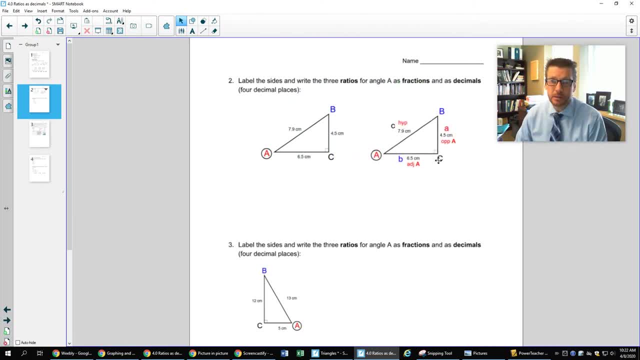 so now we have opposite adjacent hypotenuse labeled and the number is in little a, little b and little c. today we're more worried again about which ones are the opposite adjacent hypotenuse, more so than a, b and c. so the next thing you want to look at again is what were 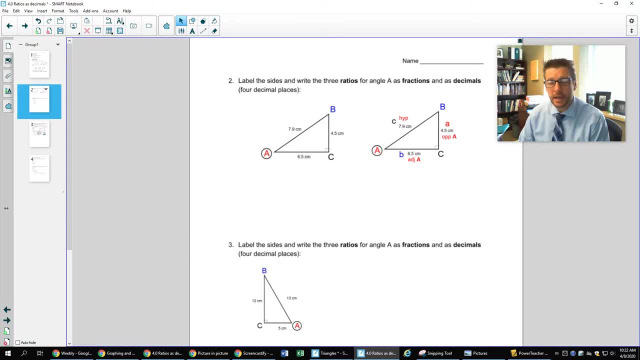 the definitions of our, of our ratios, and then how do we put those into fractions and then how do we change those to decimals. so i'm just going to grab again and some information that i have done. i'm just going to copy and paste that in here and then again, if we're going a little quick, just 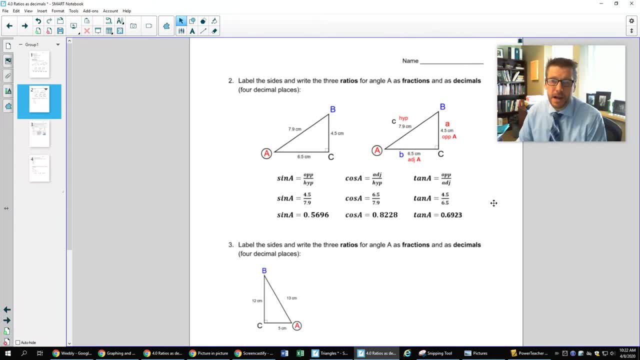 please press pause or replay the video and come back to this information. we want to know that sine is always the special ratio opposite over hypotenuse, cosine is the special ratio adjacent over hypotenuse and tangent is a special ratio, ratio opposite over adjacent. so again we're going. 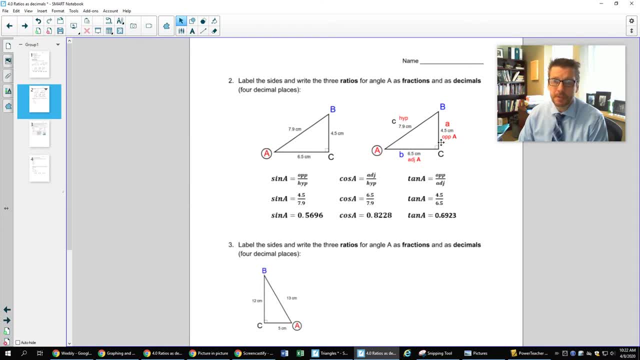 to go back to my triangle and instead of writing opposite, i write 4.5, instead of writing hypotenuse, i write 7.9, and i repeat that for my three special ratios. and then the last thing i want to do is i want to take each of these fractions and i want to turn them into decimals, so i want to go four. 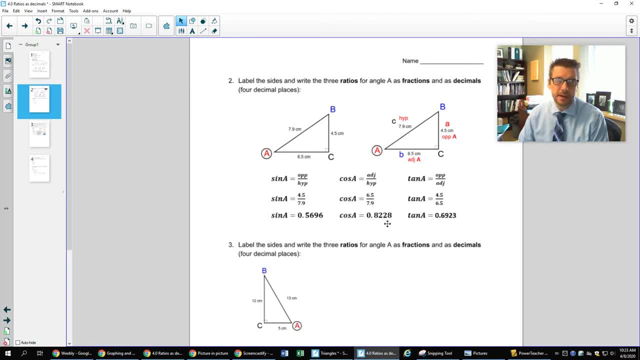 and a half divided by 7.9. i want to go 6.5 divided by 7.9. i'm going to go 4.5 divided by 6.3. and again what i've done with all my answers, as i've rounded them off to four decimal. 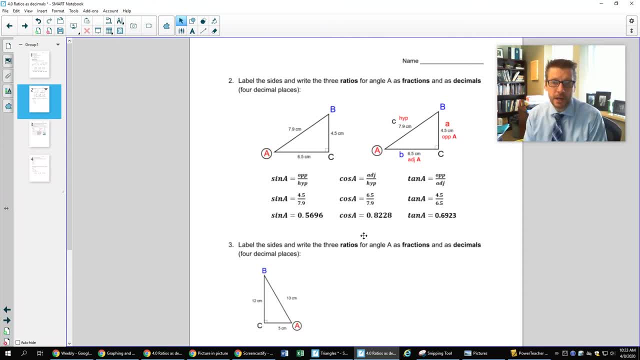 places. if you don't have the last number right because of a rounding error. that's a pretty minor error when you get that far into the ratio. so that's that's what we want to do. we want to know that we can label triangles still and that we can write our three special ratios as fractions. 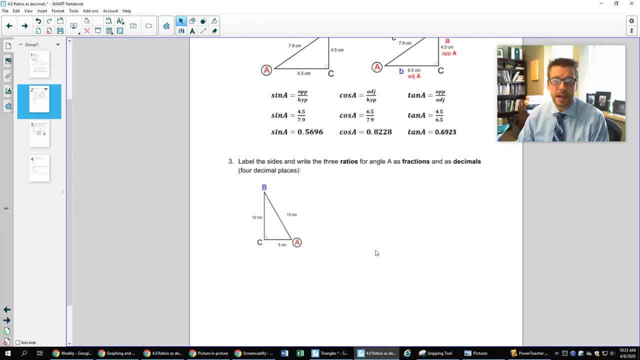 and as decimals. so let's let's do one more example. so this was about example a. question one was about was about angle a. so question three again, i'm just going to grab some work that i have done over here labeling the size adjacent opposite hypotenuse. i want to take and make sure that i 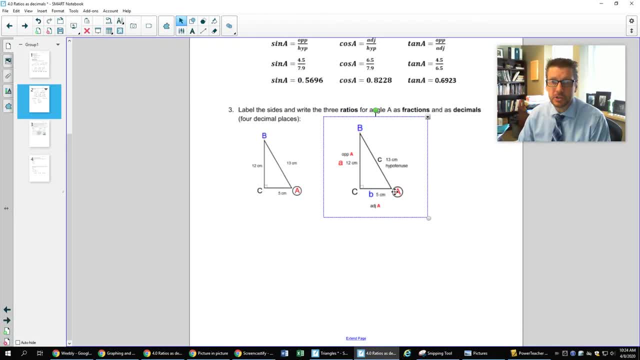 have the skills, first of all, to finish labeling my triangle, or to label my triangle. a opposite of a is little a c right angle. opposite of the right right angle is the hypotenuse. and if i've got opposite and hypotenuse, that means the bottom side here must be the adjacent side. 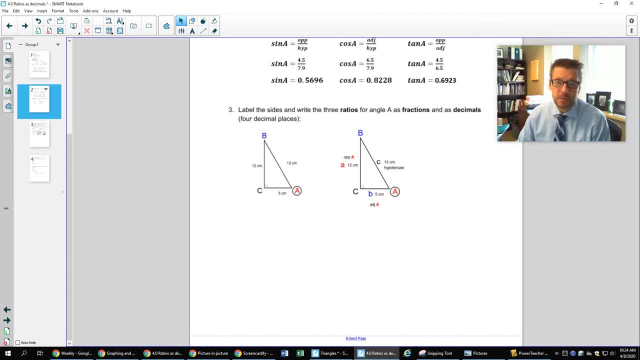 and then i want to just review what my three ratios are, the same as they were in question, two sine cosine and tangent. i want to know that i can take all those ratios, write them as fractions. so again, i'm going to grab my, my pre-done work, i'm going to write my three ratios. 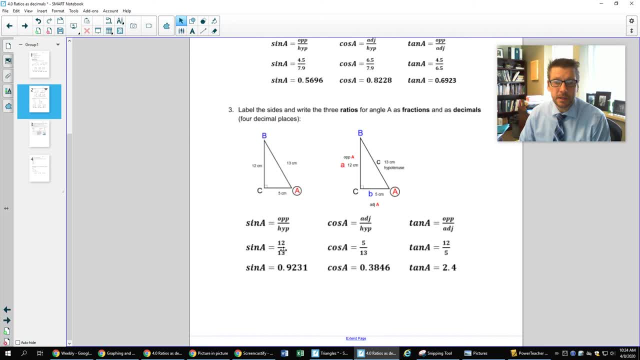 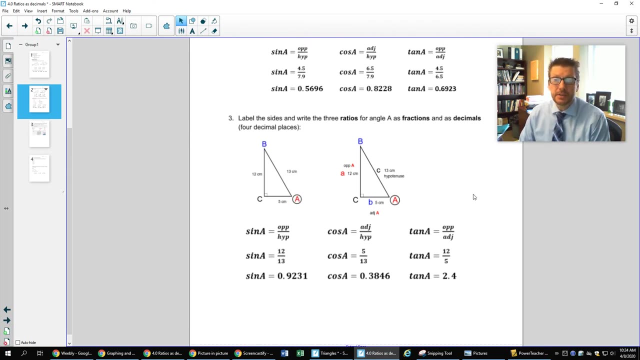 sine cosine tangent. i want to put in the ratios as fractions and want to change those ratios to decimals. it's a little bit different. this time tangent is 2.4. it didn't round off to four decimal places so i just left like that. okay, so that's, that's kind of a key. 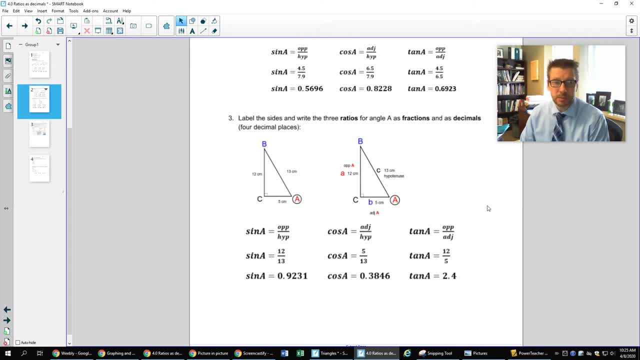 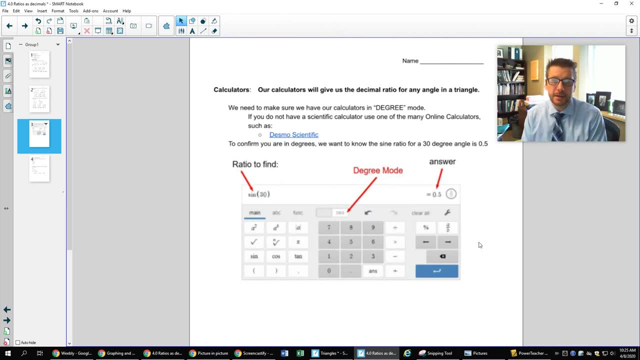 thing for our lesson is understand that we can do fractions as decimals. the. the next page here just talks again about us being able to work a calculator because every angle in a triangle except for the 90 degree angle. that one's kind of a different little situation there, but the 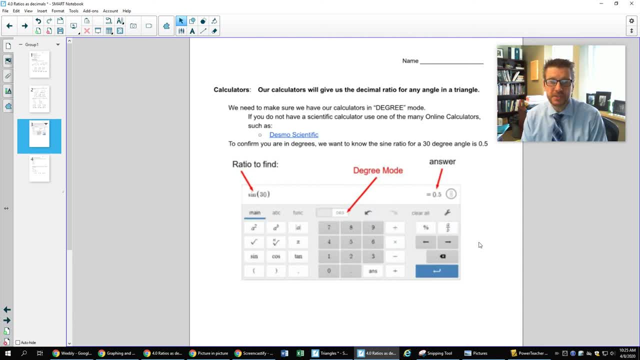 small angles, the acute angles in the right angle triangle, all have sine ratios, cosine ratios and tangent ratios to them, so we need to work with a, with a scientific calculator, though, so the online calculator that i've linked in our lesson is the desmos calculator, and that's a handy one. 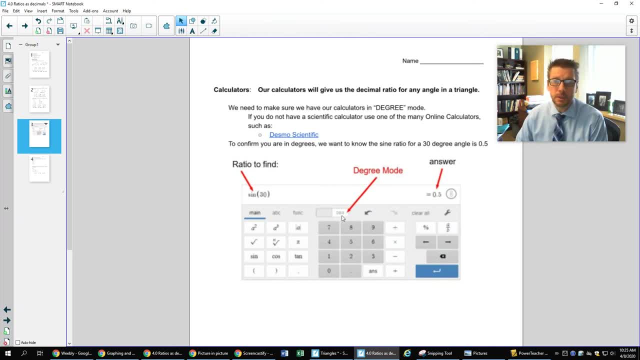 please make sure it says degree. so you're working in degree mode. uh, and then if i want to do the sign ratio, just do a quick check that i know i'm in degree mode. i would just press sign. sign pops up and then i'm going to put in the 0.5. so i'm just going to maybe do that here quick. 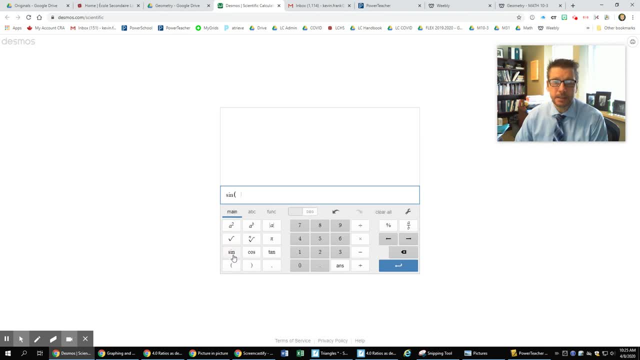 it's going to grab the calculator. uh, sine of 30 and equals 0.5, and if the answer shows up, unless i do more work, i need to press enter. so, sine of 30 degrees, sine of 30 degrees is 0.5, so i know. 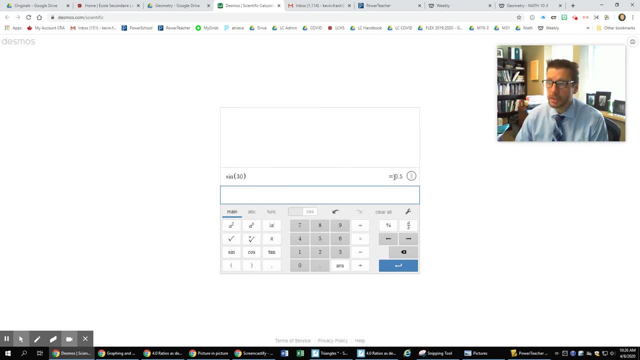 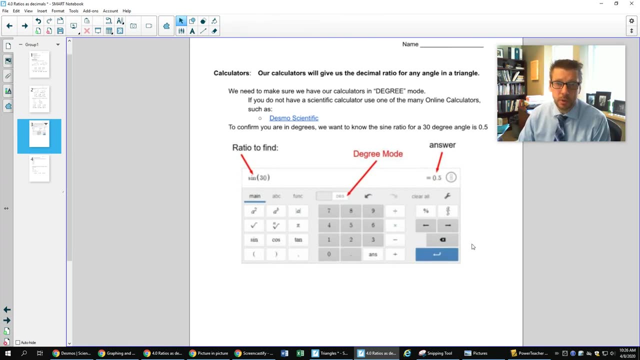 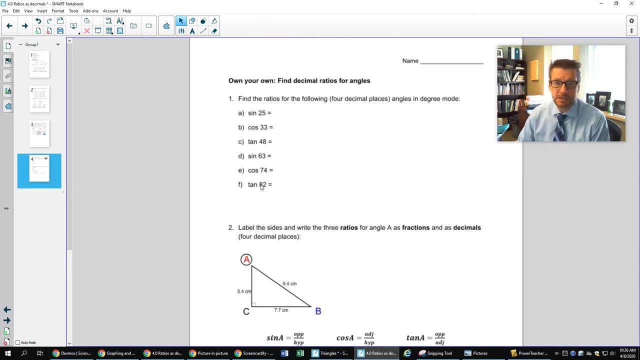 that my calculator now is is in degree mode and that's that's important to me. so that's, make sure you're working in the calculator and make sure you know you're in degree mode and that's it for the lesson you. you are now able to kind of try just taking these eight questions here. these are all degrees. 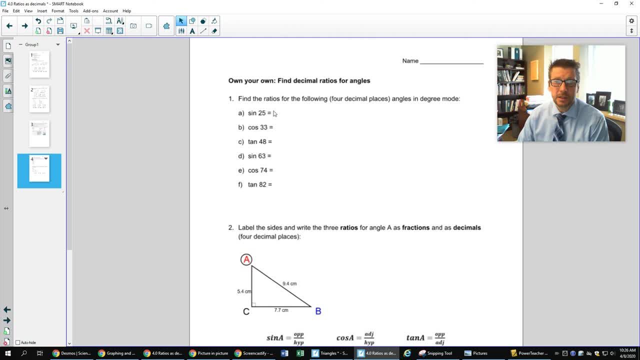 just make sure your calculator is in degree mode, find each of these ratios to four decimal places and then, on question two, just like we did on our first three examples, label the size of the triangle opposite adjacent hypotenuse and then write your ratios as fractions and then change those to decimals. and that's it for the week. hope you guys had a great week and 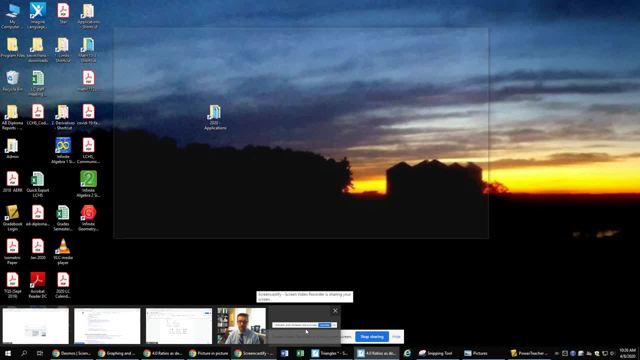 we'll see you guys next time. bye, bye after easter. hopefully the easter bunny is good to everybody. take care. 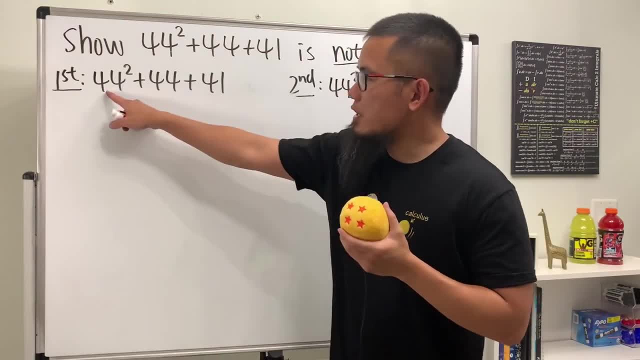 Two more ways of showing this is not prime. Here we go From this expression. first, if you grab one from here, put it here. If you grab one from here, put it here. Everybody will have 43, right. So that's a good idea to use modular arithmetic, And we are going to write. 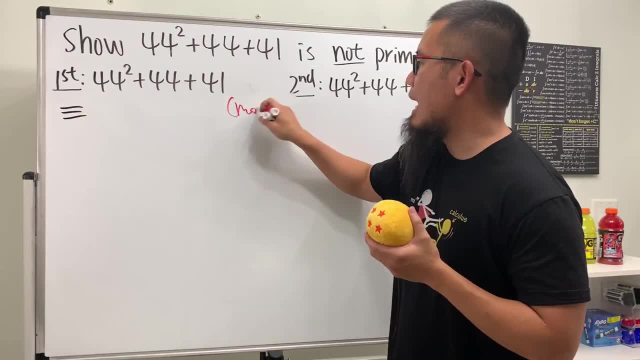 down. this is going to be congruent to the following: And, of course, we are going to do mod 43. So check this out: 44 mod 43 is going to be 1.. And don't forget the square And this. 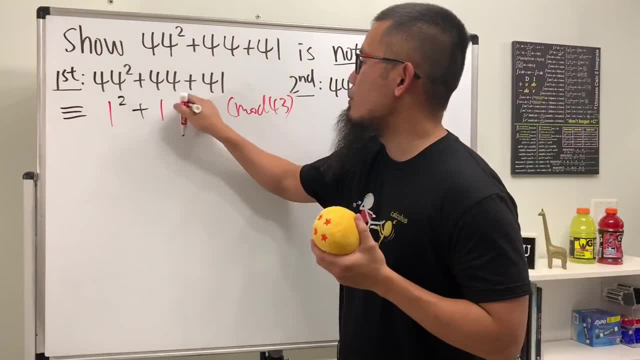 is going to be another 1.. And 41 mod 43 is going to be negative 2.. So plus negative 2, right here And now. let's work this out. This is going to be congruent to 1 squared, which is 1.. And then 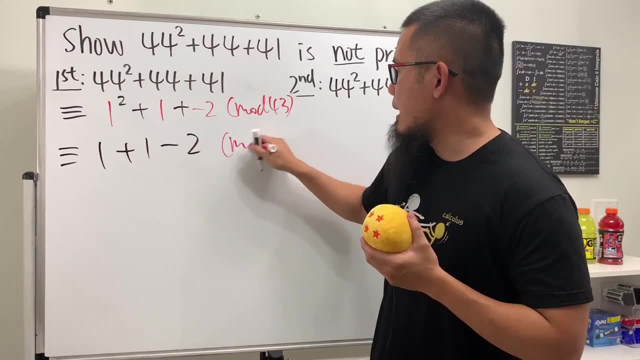 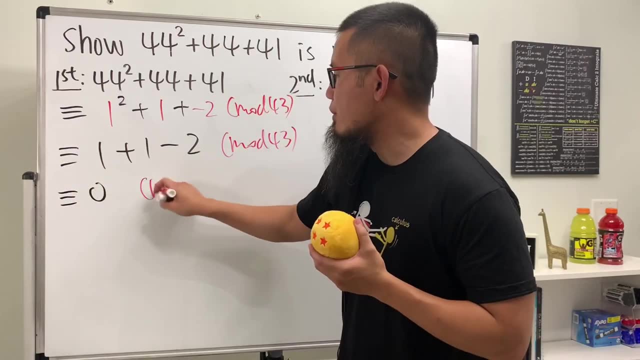 we plus 1. And then we minus 2 right here. And then still let's write down mod 43. Well, 1 plus 1 is 2.. 2 minus 2 is 0. So this right here is going to be congruent to 0. And we have to. 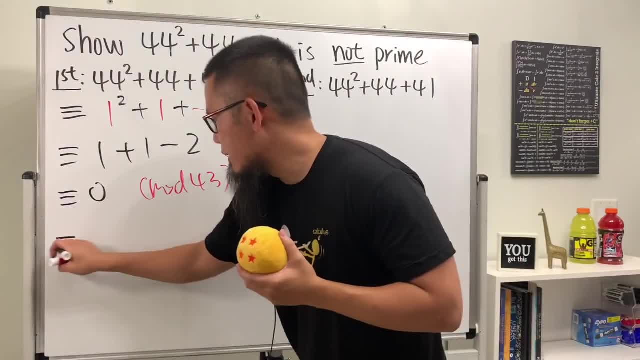 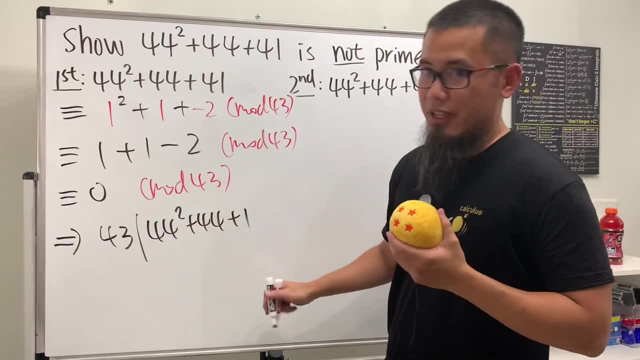 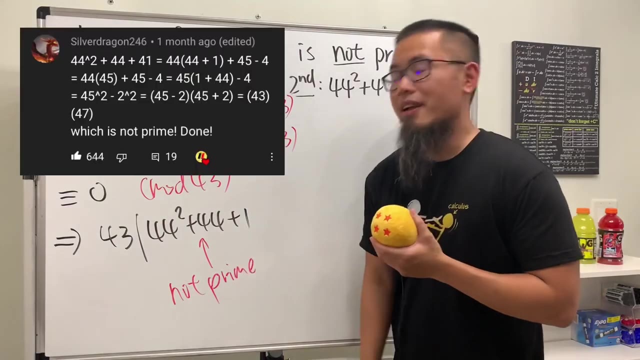 have the mod 43. What does this mean? This means the following: 43 is actually a divisor of this number, 44 squared plus 44 plus 41. Therefore, this right here is actually not prime, because we know that 43 is the factor of it, which is so nice, right, Very nice, This right here. 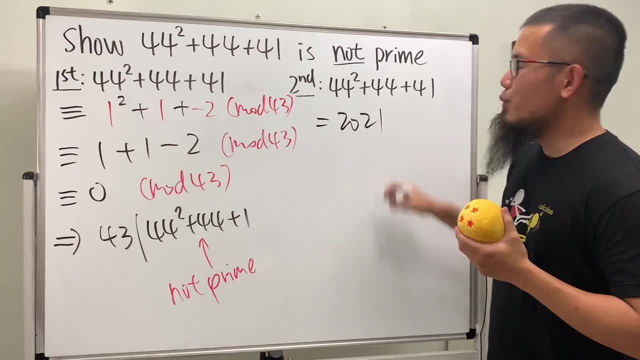 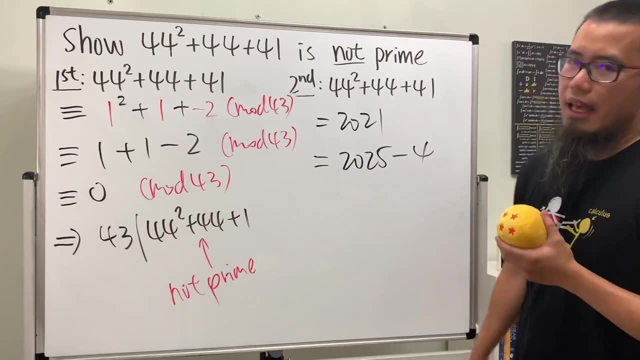 another way. If you work this out, this is going to be 2021.. This is this year, of course, And 2021 is actually the same as what? Yes, 2025 minus 4.. And this right here is yes, 45 squared, And.